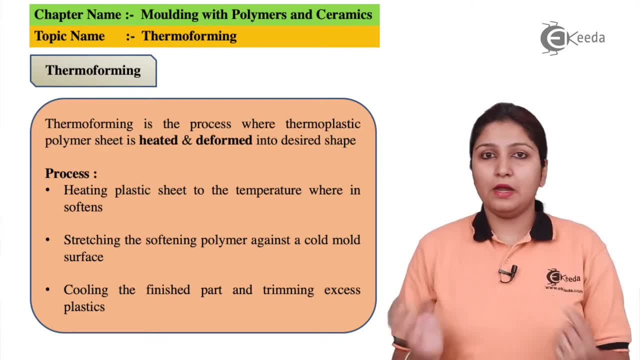 to change the shape. If the shape is changed because of the melting or because of the particles of the grain which is inside your object getting weak, it can be like your product. It can be deformed easily. So this is exact thermoforming process. So in thermoforming, 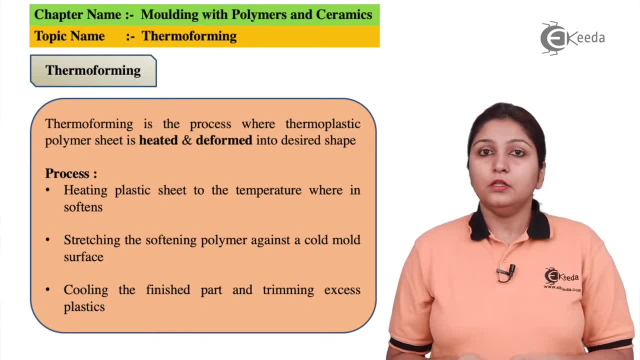 you take three steps, very important steps, in mind. The first step is your exact pressure application and pressure with heating. So pressure and heating application is there on the product. Second takes the stretching Like. stretching is nothing but deforming the product according to the need, So stretching takes place. and the third is cooling, Because 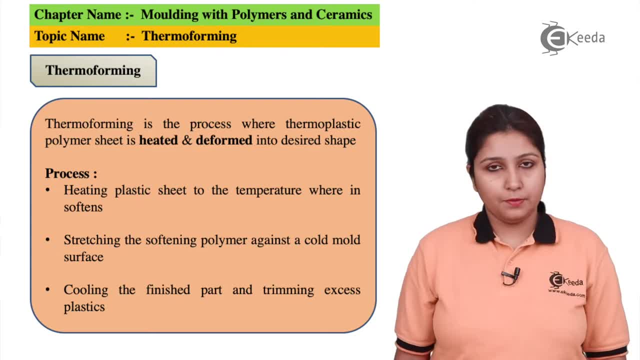 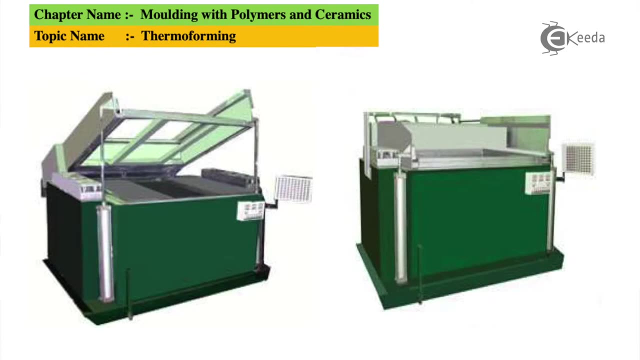 of cooling. after stretching the product, Like after deforming the product, the product can be cooled. Let the product stay in the normal environment and it gets solidified and gets the final shape. So you can see this machine. this is a thermoforming machine, where your product is getting heated and deformed. 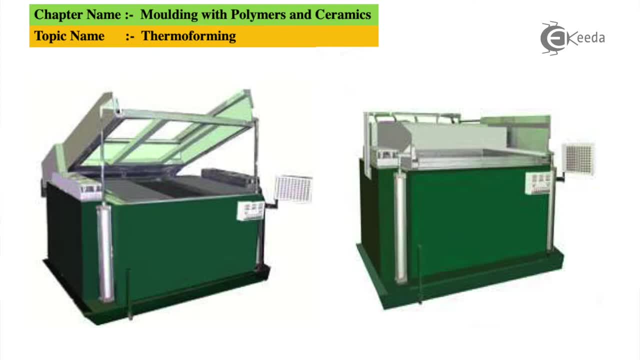 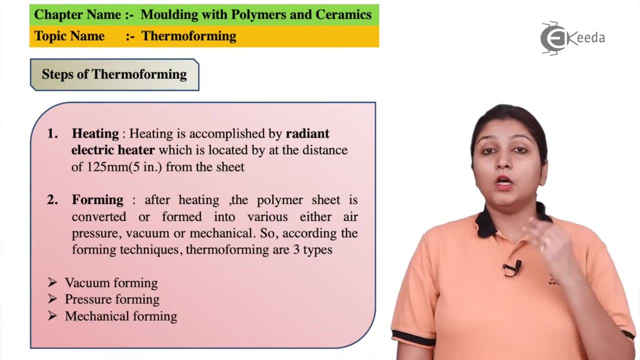 So the first photo shows the machine is open. second shows the machine is closed. So during the process of thermoforming, what happens? The product to be thermoformed, that would be the heat of plastic, is being kept 5 inch away from your exact pattern. So what happens? 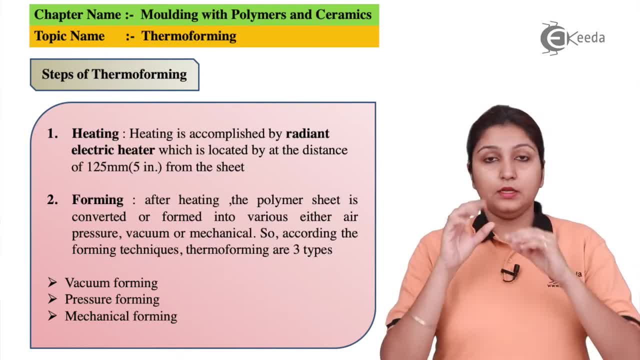 due to heating, your product, that is, your plastic, gets nearer to the object which is your pattern, and gets try to get settled on it. So in this way thermoforming process take place. Exact air or pressure or mechanical pressure is- can be used for making a thermoformed object. 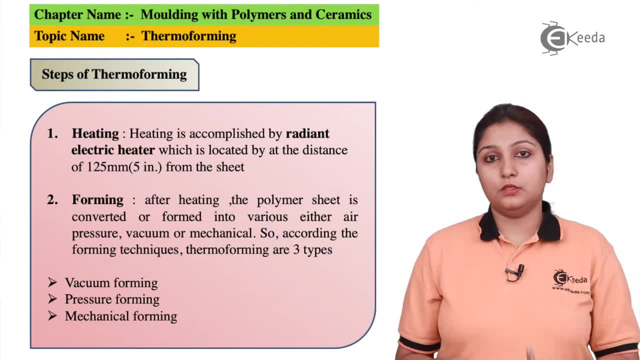 So forming takes place by these three processes: One is your vacuum forming, second, your mechanical forming and third would be your pressure forming. So these three processes, what happens In vacuum forming? you need the supply of air and a vacuum condition So that your sheet gets heated and gets settled on the object. 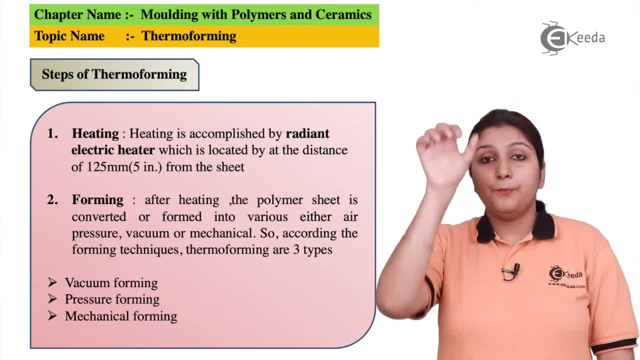 Second is your pressure forming Heated sheet is being pressurized by doing your compression process on the object which is your thermoformed object. So this is the process of thermoforming. So this is the process of thermoforming. So this is the process of thermoforming. So